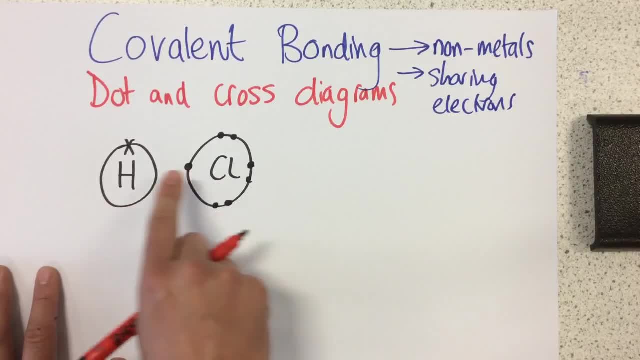 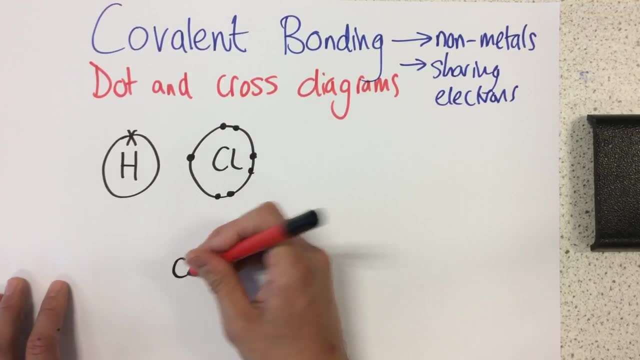 to have a full outer shell, So we can see they both need one more electron to be stable, So they bond together. and this is how we draw it. Now, what I'm going to do to begin with here is I'm just drawing the electrons that are not involved in the covalent bond on the chlorine. So there's the ones. 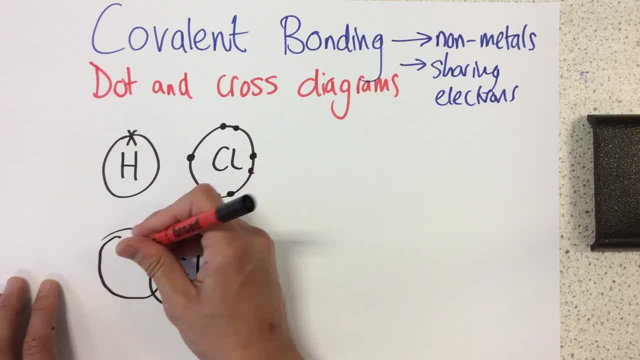 that aren't. and here's my hydrogen. Notice how I've drawn these two shells overlapping. Now in the middle, I'm drawing the pair of electrons which are being shared, One from the hydrogen and one from the hydrogen. Now, in the middle, I'm drawing the pair of electrons which are being shared, One from the hydrogen and one from the chlorine. 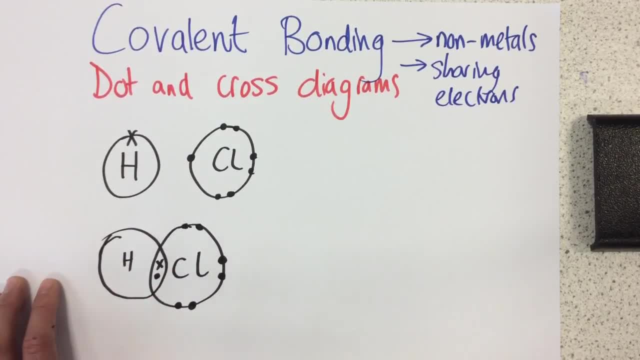 from the chlorine If we now count the electrons in each outer shell. so for chlorine, 1, 2,, 3, 4,, 5,, 6,, 7,, 8, so it's got a full outer shell. And for hydrogen- 1, 2,, it's got a full outer shell. 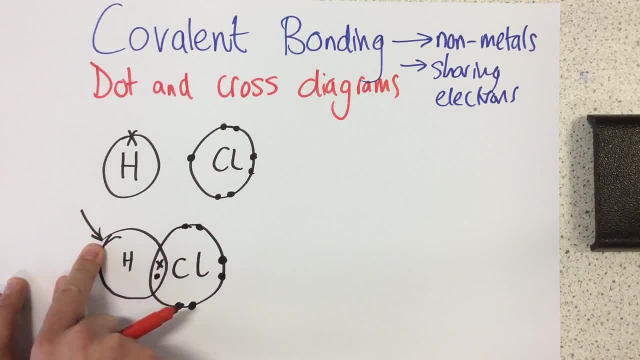 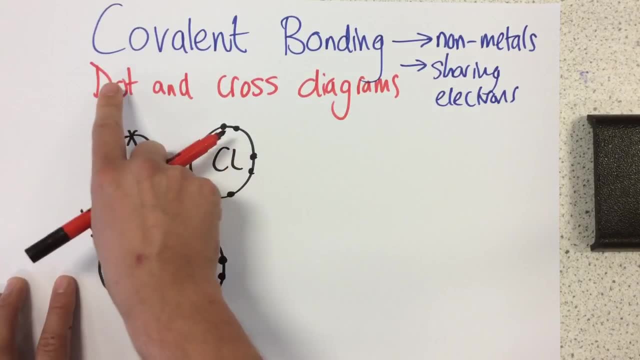 Please notice how I didn't draw the electron over here and I've drawn them in the middle, because it shows that these electrons are being shared. Also, notice the reason why it's called a dot and cross diagram. is we always draw the electrons on one atom with dots, or sorry? 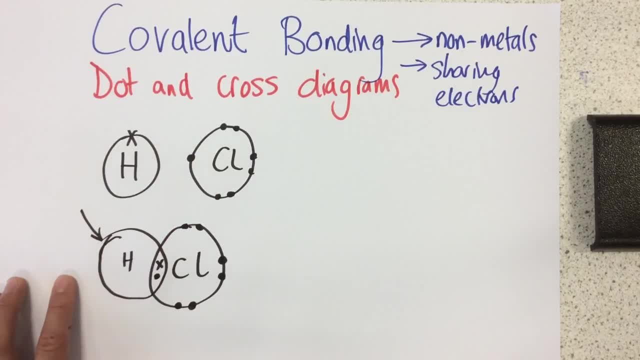 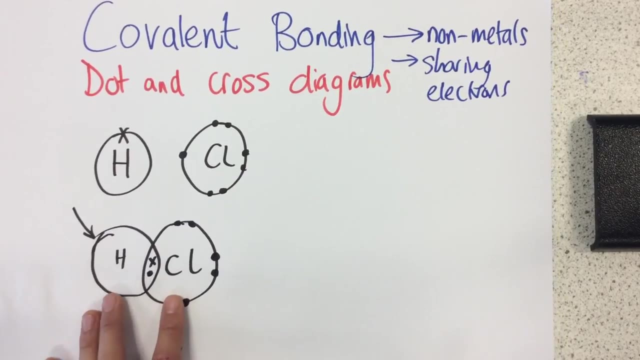 with dots and the other with a cross. This is just to show which atom they originally belonged to. They're actually both still exactly the same. They're both just electrons. So the whole point of dot and cross is just showing which atom it belonged to originally. Now the other example. 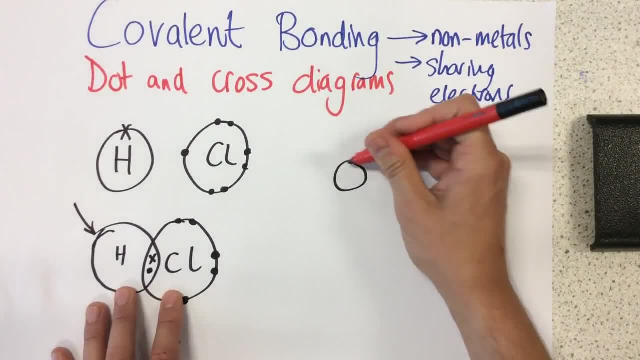 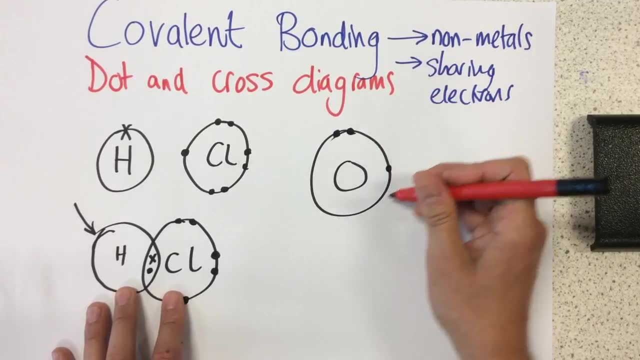 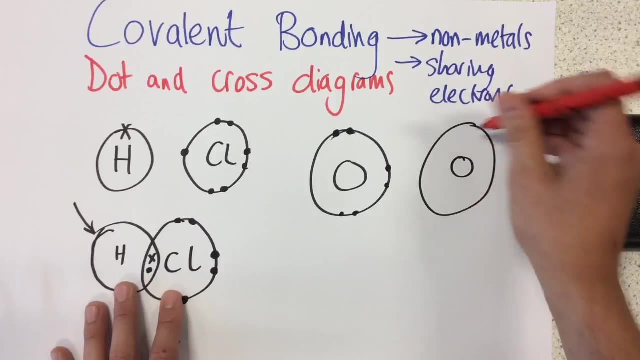 I'm going to do is I'm going to show you how to do an oxygen Molecule. So here we have oxygen which has six electrons in the outer shell. I didn't draw that very well, so I'm going to draw this one a bit better. There we go, So we can see that this 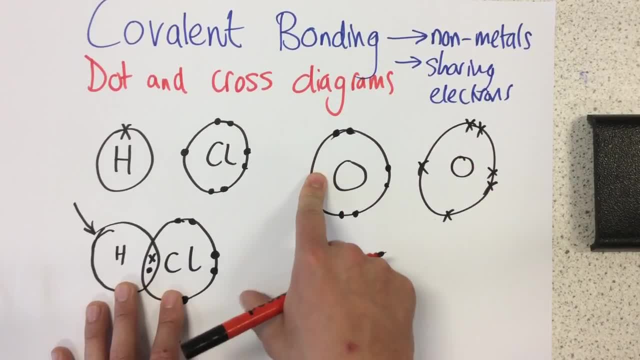 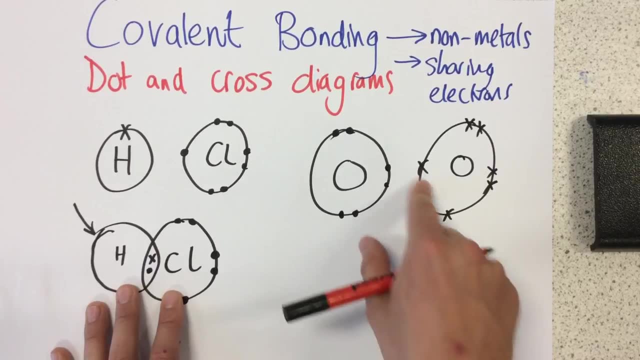 oxygen atom needs two more electrons to have a full outer shell and this oxygen atom also needs two more electrons to have a full outer shell. So they are going to share. This time this one is going to share two with this oxygen and this oxygen is going to share two with this oxygen. So let's draw them So again. 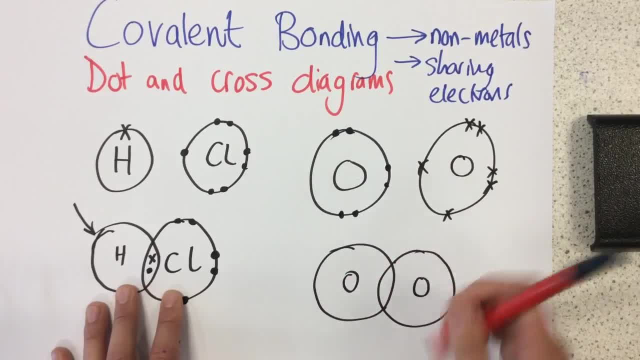 I've drawn these two atoms overlapping, just writing an O for oxygen in the middle, So we can see this time there's two of those electrons are going to be shared from this one and two are going to be shared from this one. 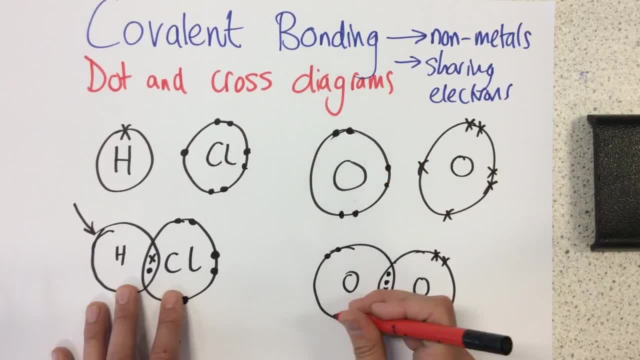 So there's just two of those electrons And these are just the other electrons that make it up. So now, if we count the electrons, we can see that this oxygen atom here now has 1,, 2,, 3,, 4,, 5,, 6, 7, 8.. 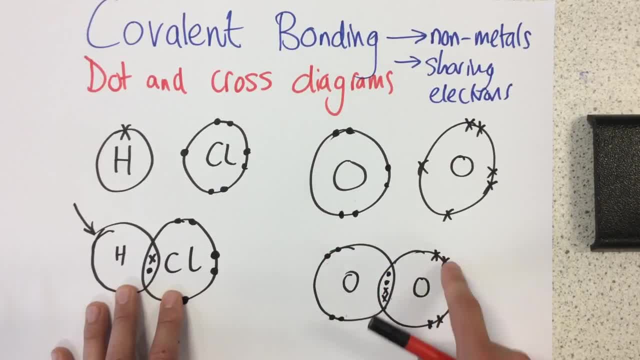 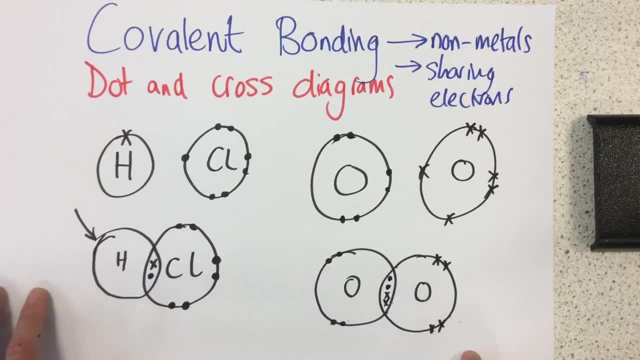 So it's stable. And this oxygen atom here has 1,, 2,, 3,, 4,, 5,, 6,, 7, 8.. So this is stable. So just to recap, the important things are: we know that this only occurs between nonmetals. 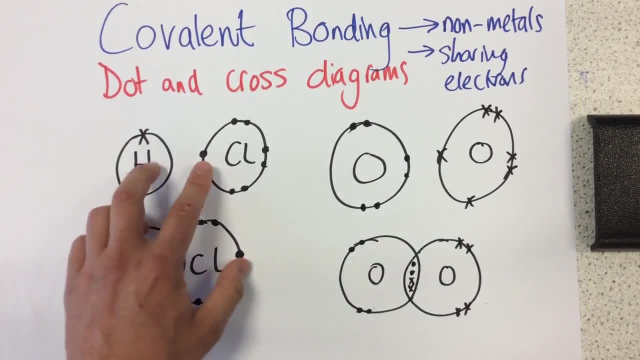 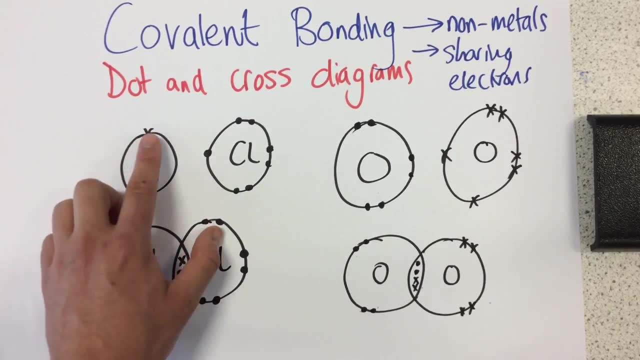 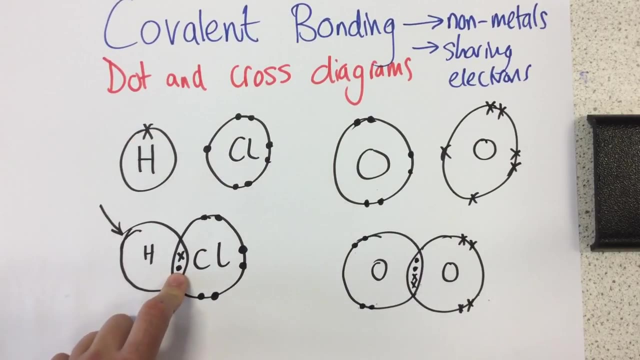 and covalent bonding is sharing of electrons. We think: how many more electrons Does your atom need to have a full outer shell? We draw the electrons from one atom with a cross, the other with a dot to show that they're from different atoms, And we draw these electrons in the middle. 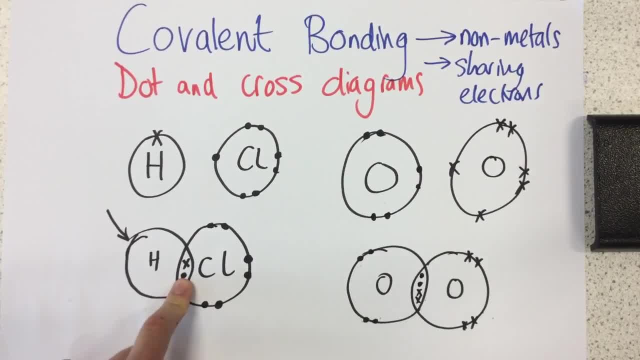 to show they're being shared. If we get all of that stuff right, we should be okay. Thank you. 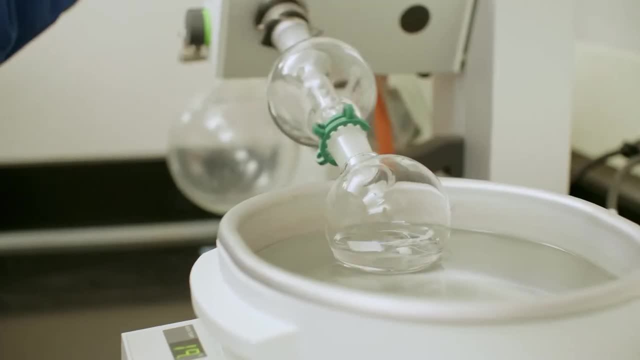 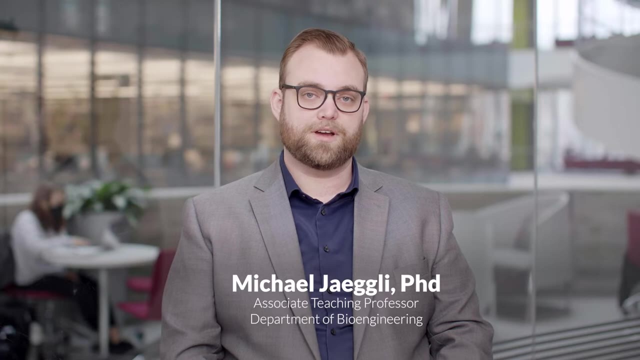 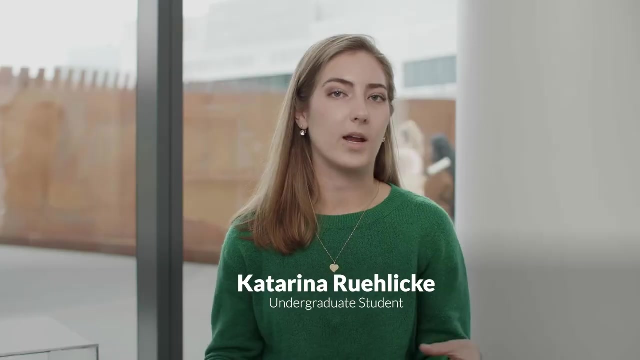 The biomechanics concentration deals with understanding both fluid and mechanical forces in the body. In this concentration, you'll study things like how cardiovascular fluid mechanics work, as well as how the musculoskeletal system functions. There's a wide range of ways that mechanics can be applied to anatomy in your biology, and that's what I like the most about.